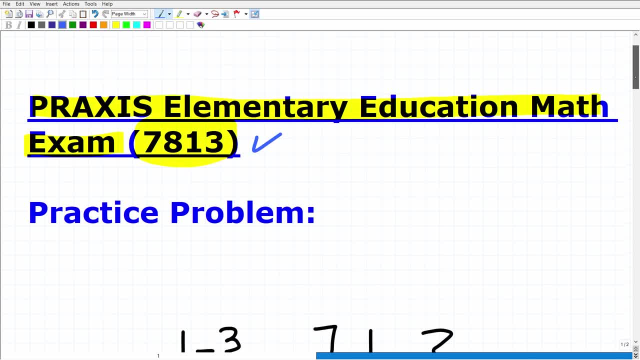 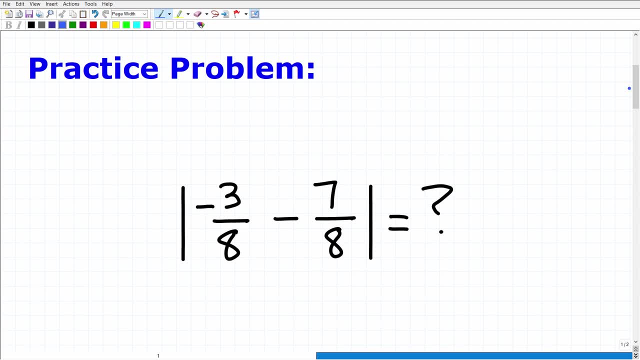 And what I have for you here is a nice practice problem that you should be able to handle without too much difficulty if you are fully prepared for this exam. So I'll kind of refrain to describe what this is, But here is the problem. Now, if you know what this is and you know how to answer this, go ahead and put your answer into the comment section. I'm going to show you the correct answer in just one second. Then I'm going to fully explain what's going on here, including a step-by-step solution. 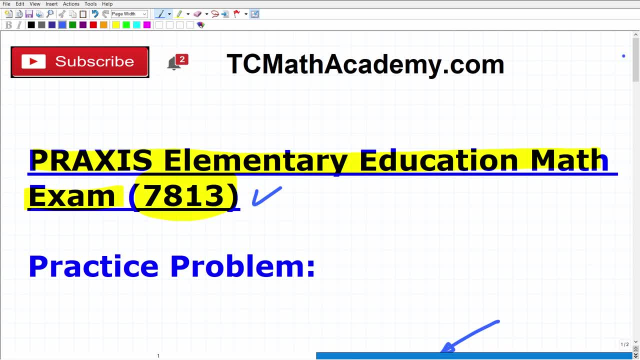 But before we get going, let me quickly introduce myself. My name is John. I'm the founder of TC Math Academy. I'm also a middle and high school math teacher. I have been teaching math for decades and I know exactly what it's like to take certification exams to include the Praxis exam. So let me just tell you something that you probably already know. 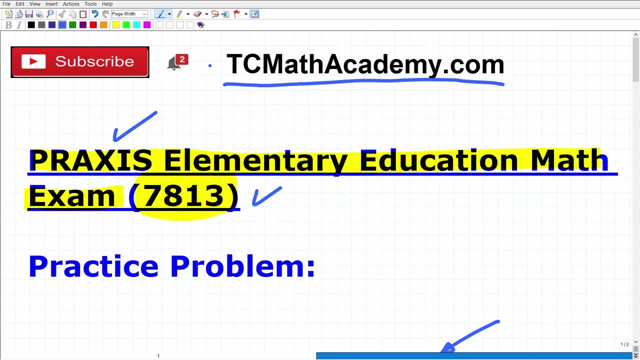 A lot of people do not pass these exams the first time out. Okay, unfortunately, it takes some people two, three, four times to pass. Now, it's my belief that everybody has the capability of passing the first time, But the reason why a lot of people don't pass the first time is because they underestimate how much math they need to know. 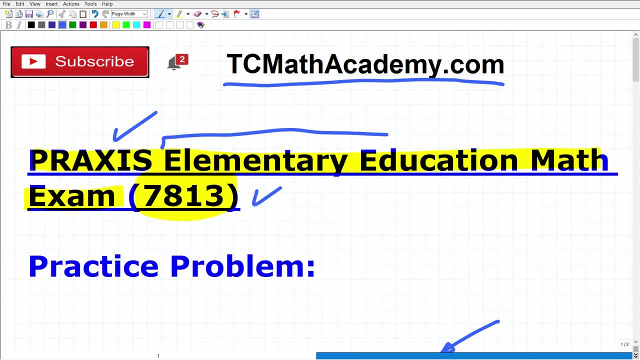 Okay, I'm here to tell you, don't let this elementary education part of the title here kind of deceive you. You need to know a lot of high school level mathematics to be successful on this Praxis exam. So if you need a way, you know. 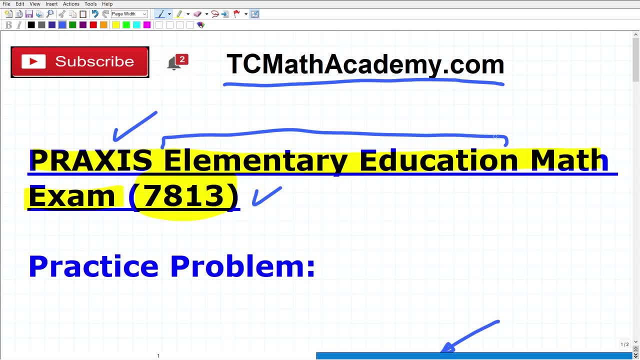 So if you're not quite sure how to study for this, but if you need a great way, which obviously you do- you need a plan to pass the exam. I have an outstanding test prep course. You can find a link to that in the description of this video. that will help you get fully prepared for this particular Praxis exam. 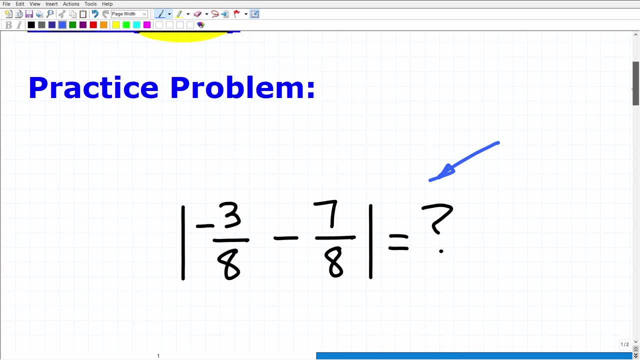 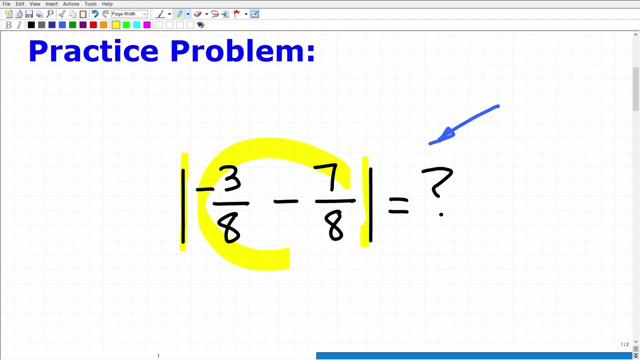 But let's go ahead and get into this problem now. So what are we talking about here? Well, we're talking about an absolute value problem, Okay, so we want to find the absolute value of all this stuff right there, And what is the answer? 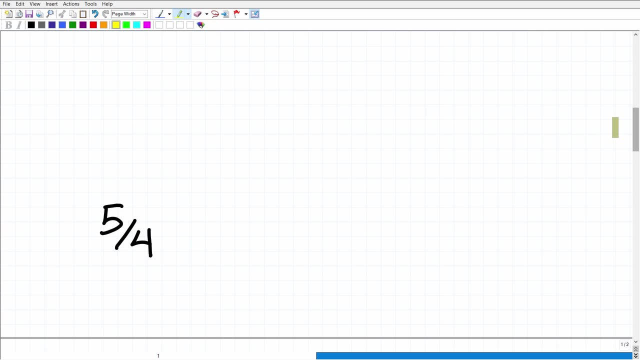 Let's go take a look at that right now. The answer is five-fourths. All right, So again, this is a very easy problem. Now, if you didn't get this right, don't panic, Just use this as feedback. 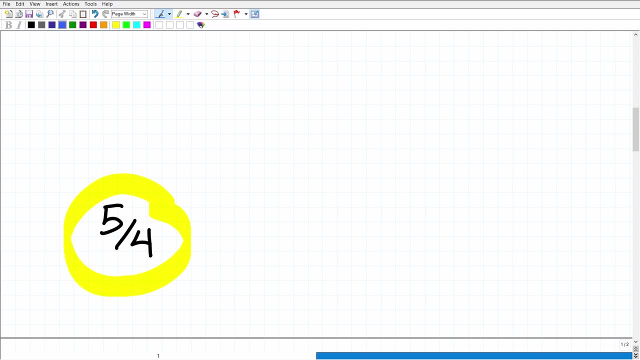 And if you did get this right. this is by no means any indication that you're fully prepared, But that is still a nice job. Now here's the deal, right? We are talking about absolute value, So I'm just curious: What is the definition of absolute value? Can you answer that? 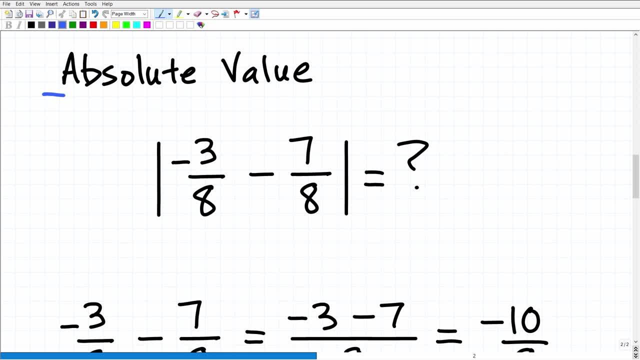 Well, hopefully you can, because That's something you should definitely know for this particular Praxis. but let's go ahead and get into the actual mechanics of this problem, All right. So the first thing we need to do is we have to simplify this kind of problem inside the absolute value. 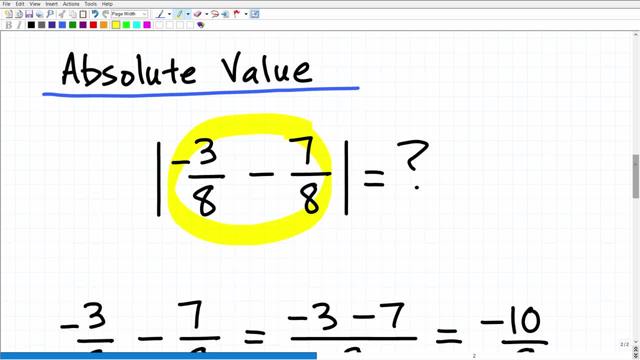 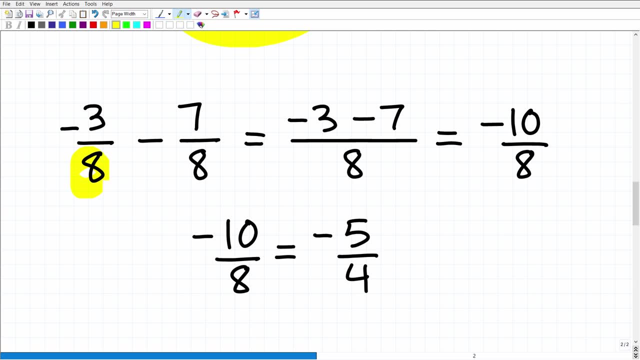 So we have negative three-eighths minus seven-eighths. So we're talking about subtracting these two fractions. This is super easy. Remember, when you want to add and subtract fractions, if the denominators are the same, all we need to do is: 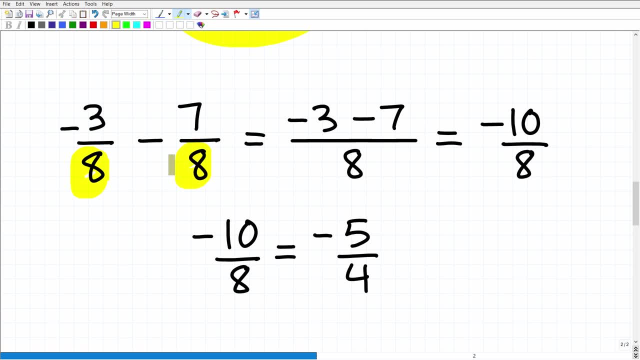 add or subtract the respective numerators. So here they are the same. So we have eight as our denominator. So we're going to subtract negative three minus seven and we can see that right there. So negative three minus seven is of course negative ten, and that's going to be over eight. 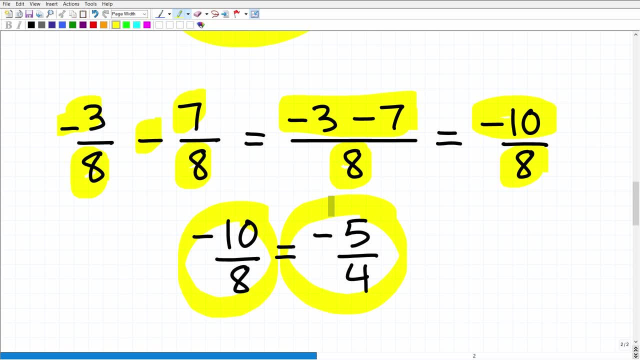 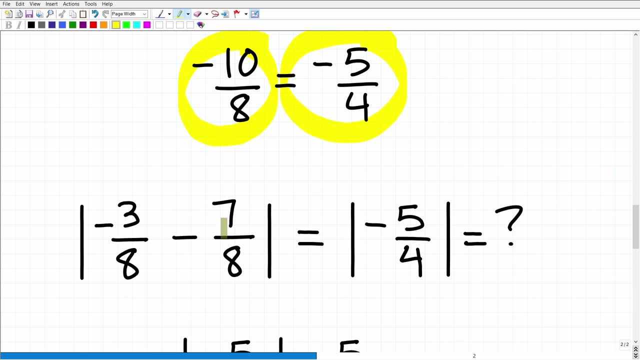 Okay, so negative ten over eight. We can reduce that fraction down to negative five-fourths, Okay. so that really makes our problem the following: Okay, we're taking the absolute value of all of them, All of this, we did that math and that now is negative five over four. 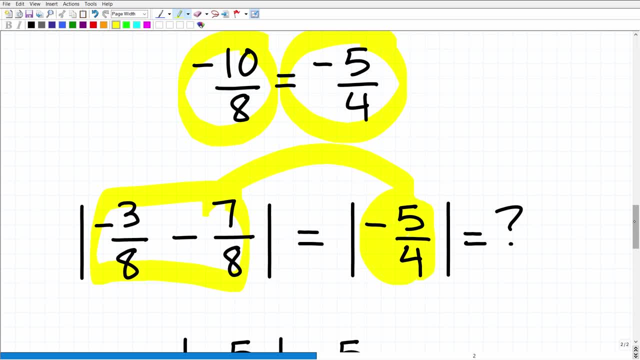 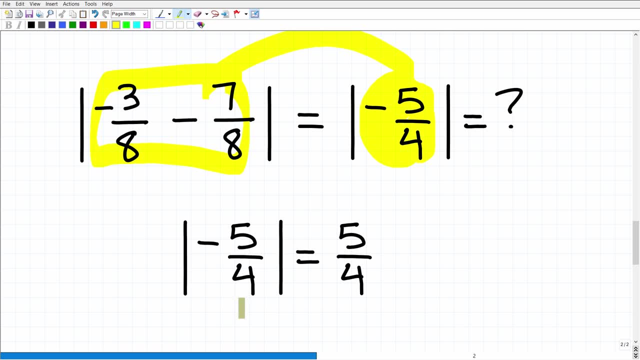 So what is the absolute value of negative five over four? Now, most people don't have a too difficult time answering basic absolute value questions like this. They'll just say, oh, it's just the positive of this number. So if this is negative, it's always positive. If this was positive, this would be positive. 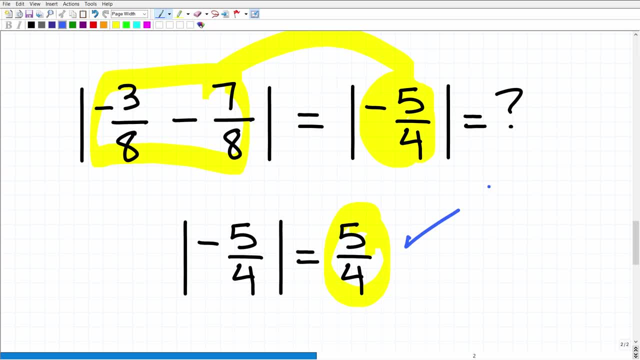 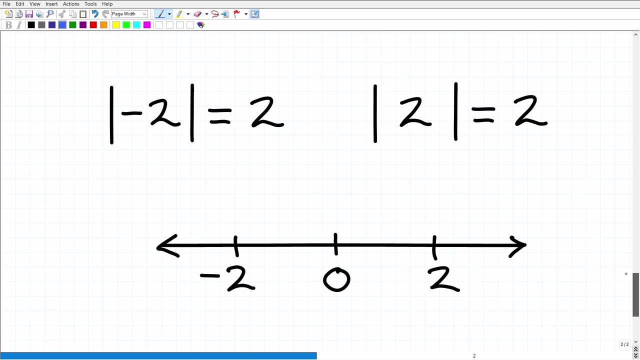 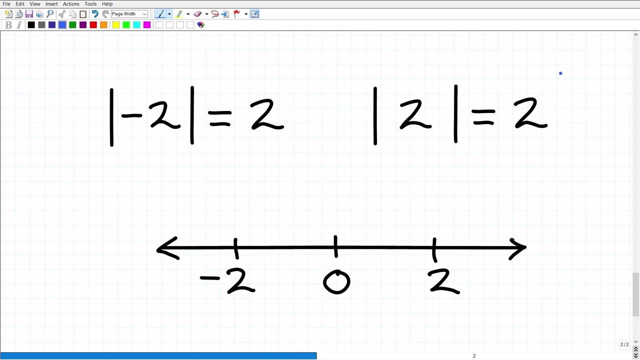 And that is correct. So this is how you answer the question. but really, what is absolute value? Let's go ahead and just quickly review. Let's review this right now. So absolute value is the distance a number is from zero. Okay, so here let's take a look at this right here first, 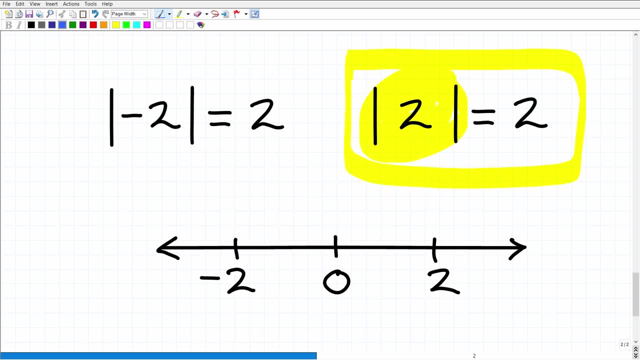 So when I look at absolute value you kind of really think about like being asked a question: Hey, how far is two from zero on a number line? That's what absolute value is right? So of course, the absolute value of two is two. 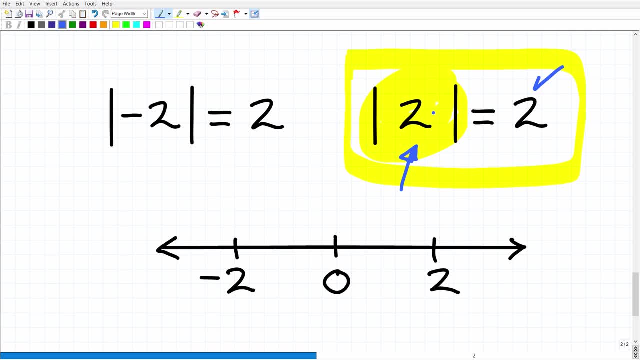 So it's saying: hey, the distance, The distance from two, from zero on a number line, is two. So we can kind of see that visually here. So here is zero, Here is two, The distance is two units. So in other words, if you had like a, you know, a roller or a tape measure, right, you would kind of measure. 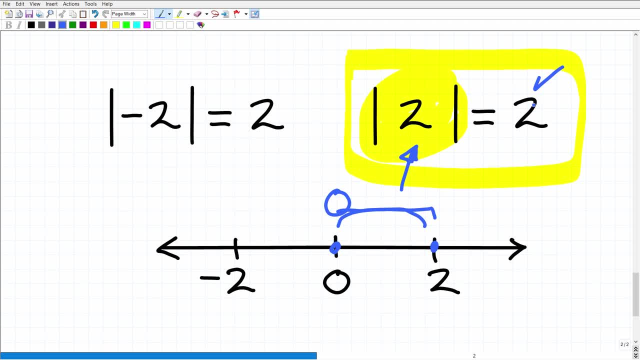 You kind of go out there: Oh, that's two units away from zero, No problem, Okay, so two is two units away from zero. All right, now let's take a look at this one here. this problem, So the absolute value of negative two. 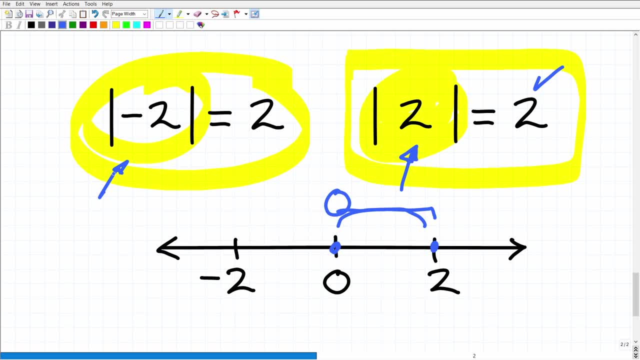 Well, again, this is asking: How far is negative two from zero? Okay, so of course we know the answer is two, But you can kind of see visually that the distance is the same, right? So negative two is in fact two units away from zero. 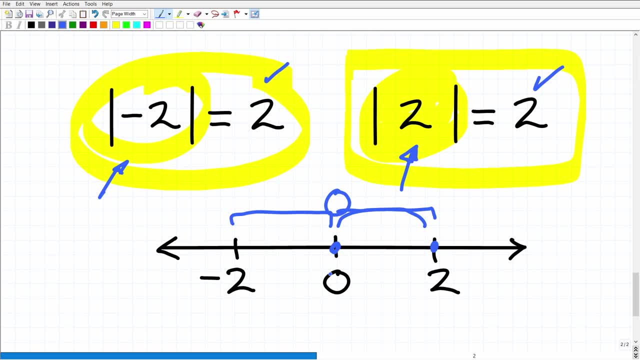 Anytime you're talking about distance in general, you're talking about positive units, displacements, right? You're not talking like I'm going to go negative 80 miles down the road, Although there is, you know, times where you do think of negative values in terms of displacement and distance. 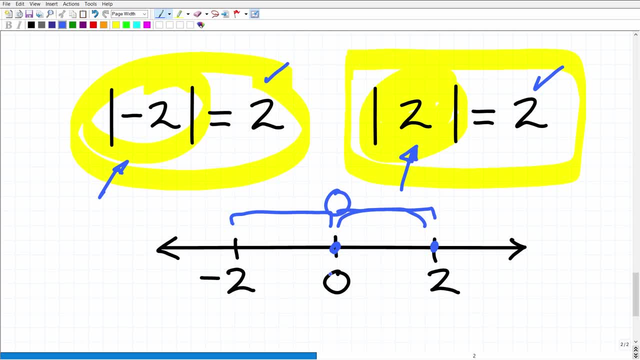 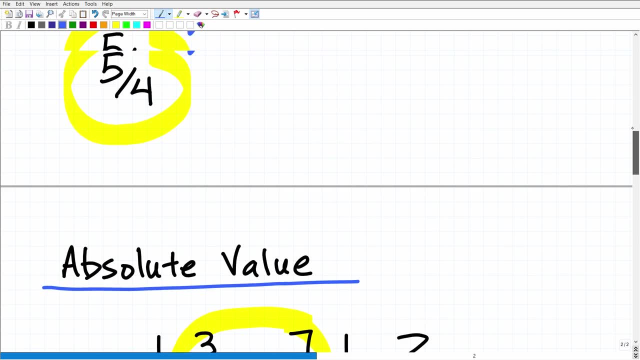 But when it comes to absolute value, just remember it's always positive right. Distance from zero is always going to be positive. All right, so hopefully this was pretty easy stuff Again, don't you know? take this as an indication of you know, this is like the hardest stuff that you'll see on this particular practice. 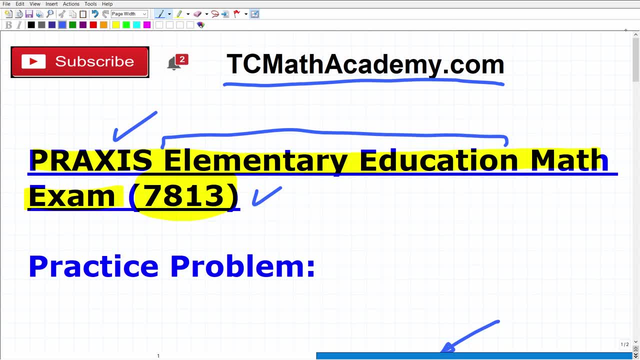 Again, you're going to have to know a lot of mathematics to pass this thing the first time, And that is what I'm going to encourage you to do. So again, if you are struggling or if you're kind of, you know, don't have a fully organized. 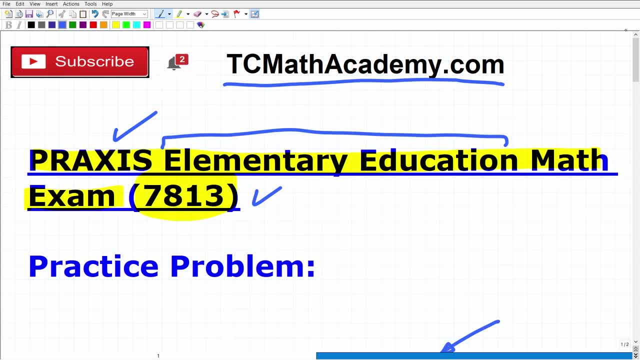 organized plan to study for this particular practice. check out my test prep course Again. you can find a link to that in the description below. It will really really help you out. Okay, so, with that being said, I definitely wish you all the best on this particular practice exam. Thank you for your time and have a great day.